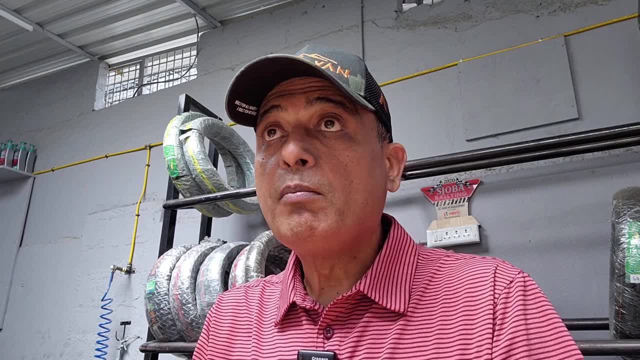 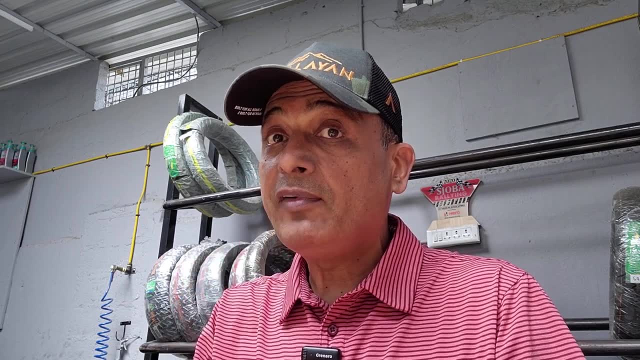 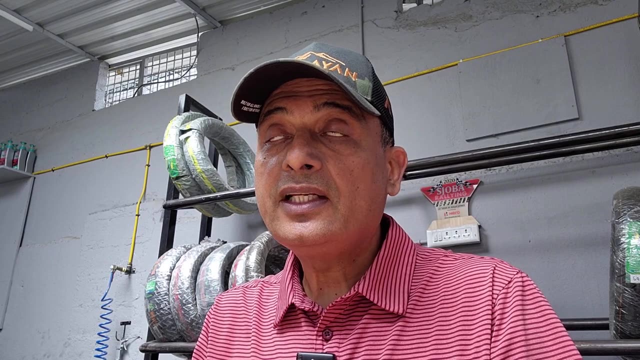 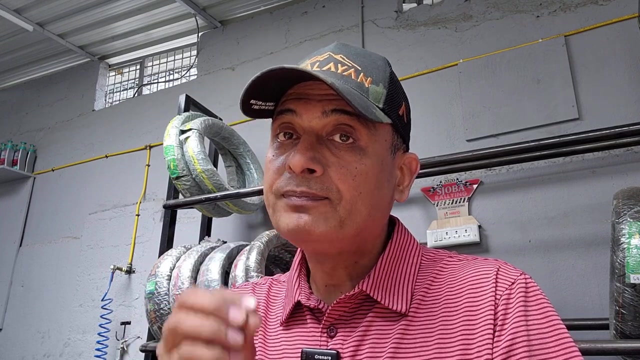 Maintain the correct tire pressure. Tire pressures are the most ignored item in maintenance and can drastically affect mileage. Check tire pressures every week. Ensure a clean and lubricated tire. Ensure a correctly adjusted chain. The chain can sap power. It can create so much of friction and drag. the mileage can drop drastically. Every 500 kilometers clean and loop the chain. 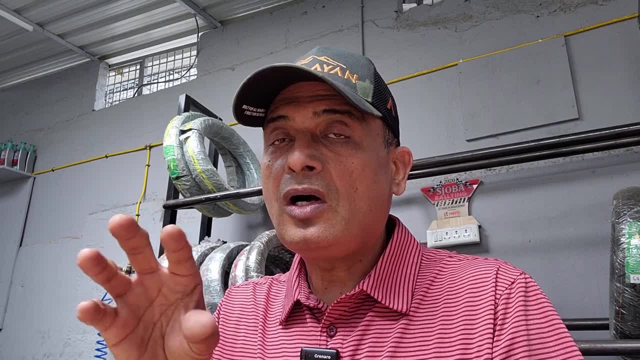 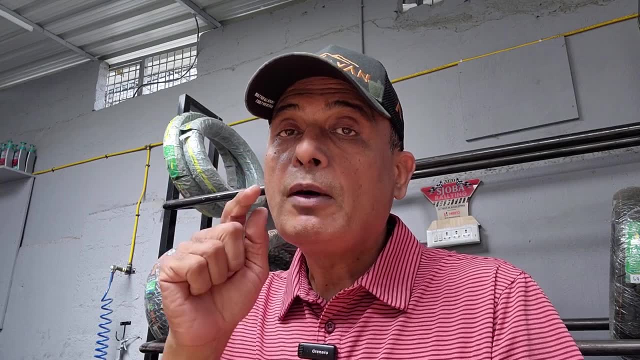 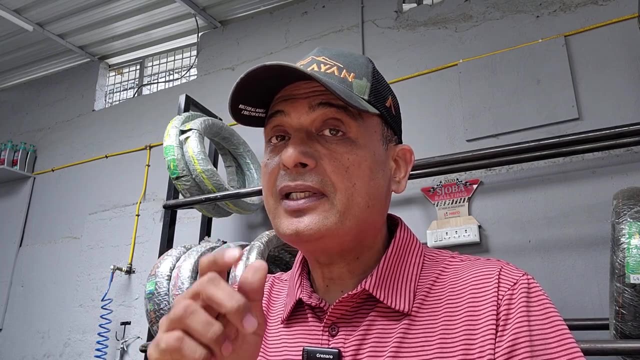 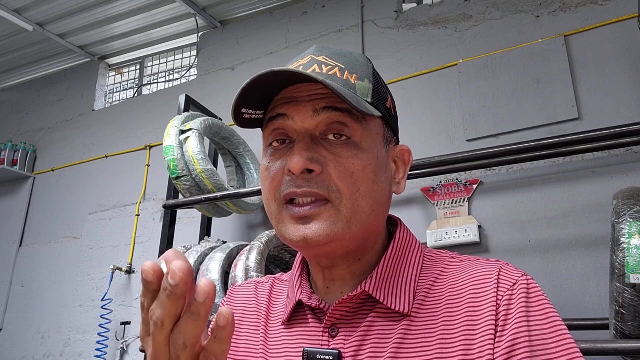 Less electrical accessories: Fog lamps, horns, all those blinking fancy lights- they all consume power from the alternator. More load on the alternator, less the mileage. Timely and correct setting of valve gaps As per manufacturer recommendation. please get the valve gaps checked. It can be 10,000 kilometers or 20,000 kilometers depending on the brand. This will help the engine run efficiently. 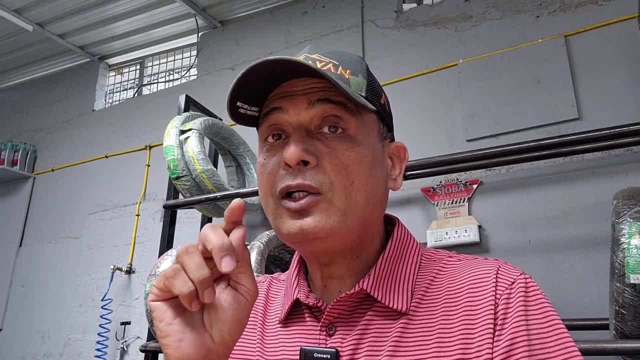 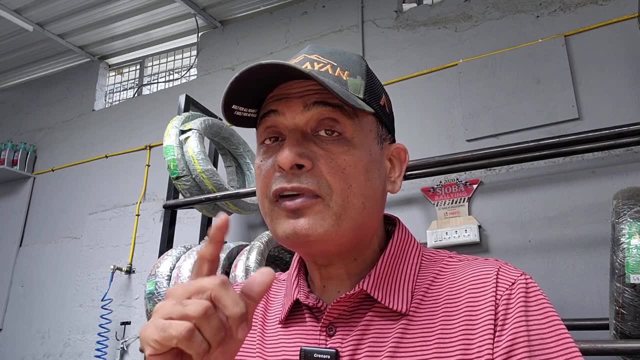 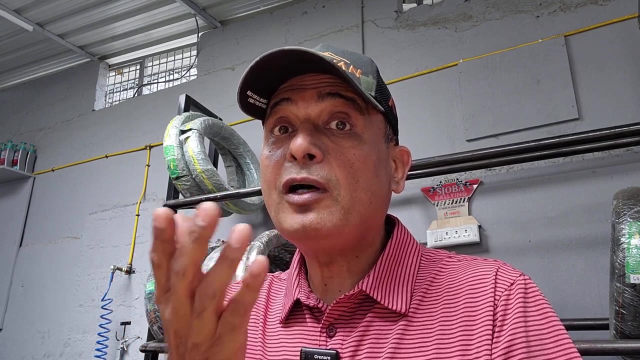 If it is a liquid-cooled engine, ensure you change the coolant on time. A good coolant ensures the correct operating temperature. Also, it reduces the fan from coming on too frequently. When the cooling fan runs, it's taking more power from the alternator, which again takes the power from the engine. 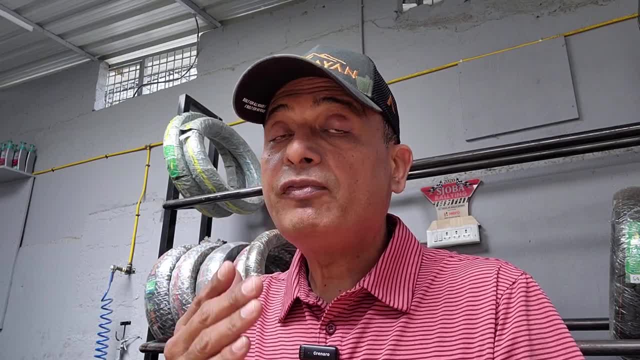 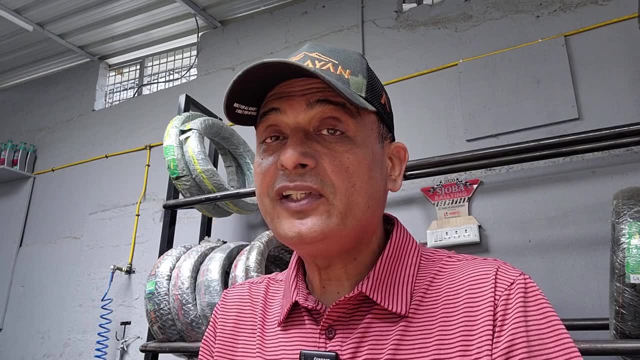 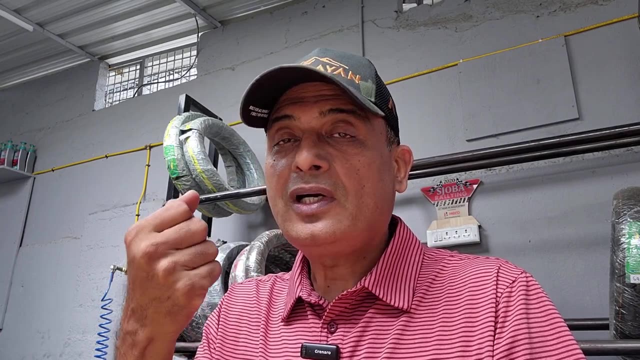 Keep the coolant in good condition. Timely shifting of gear. Do not over-rev, under-shift. Going slowly does not necessarily mean better fuel efficiency. There is an optimal speed, so shift gears accordingly. Throttle application: be gentle, Do not slam the throttle open. 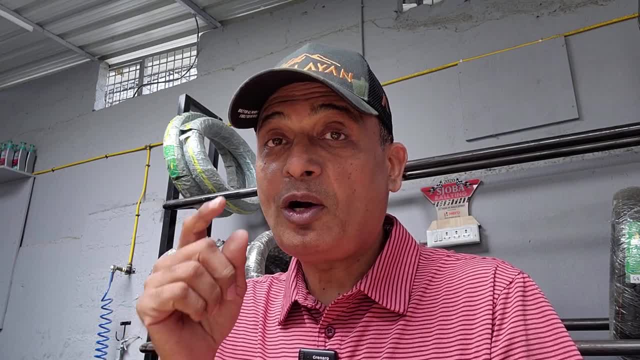 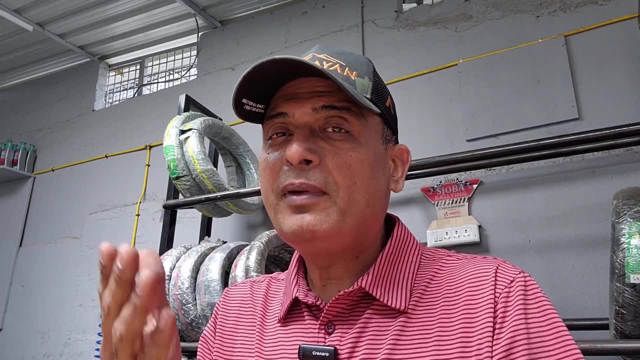 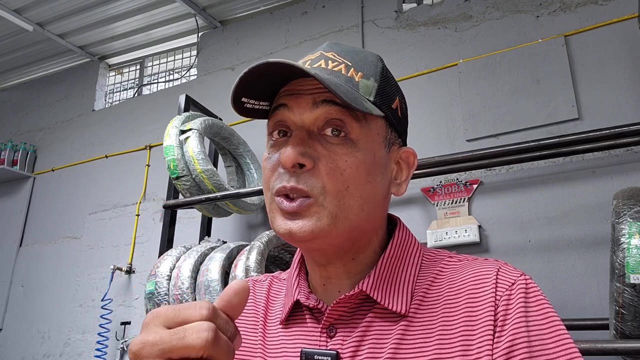 Acceleration is the biggest enemy of fuel efficiency. Roll on, roll off When stopped at a signal. if it's going to be more than 30 or 40 seconds, switch off. Start it when 5 or 6 seconds to go to green. 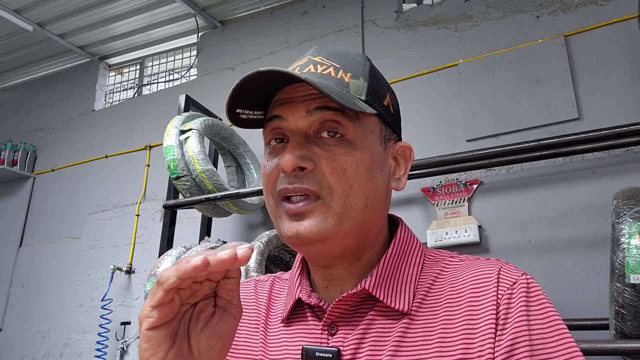 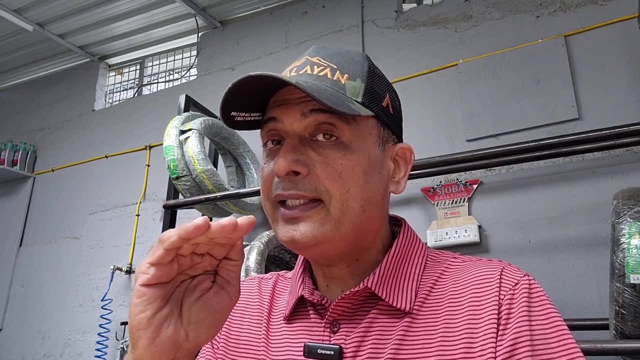 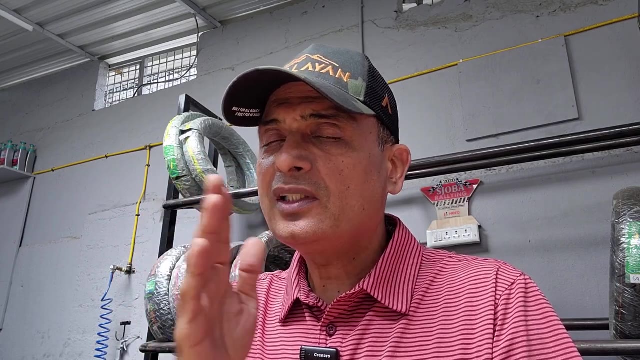 And always check mileage full tank to full tank. Do not rely on the fuel gauge or the light, They are just a rough indication. Fill the tank, Run about 200 kilometers, come back to the same bunk, same pump. Do it a couple of times because traffic conditions can vary. 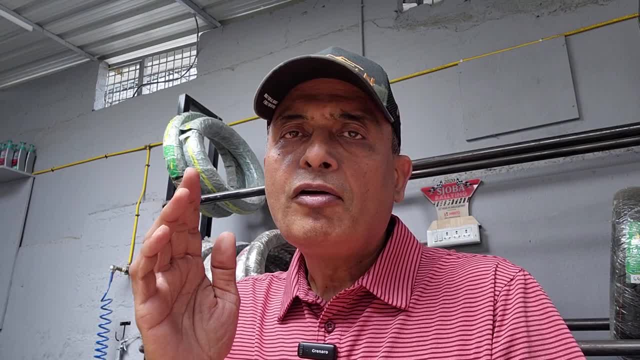 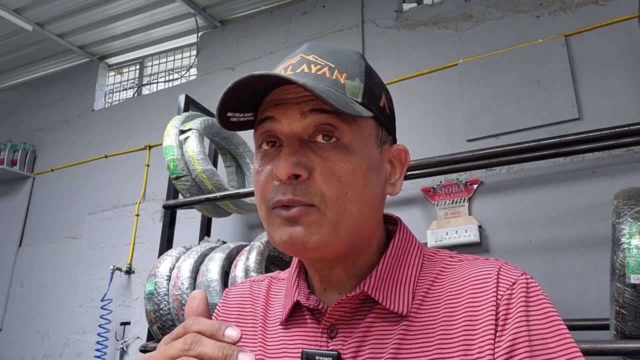 So this is the best way to know the true mileage. Follow these and I assure you you will get better mileage from your motorcycle. While all of it is not possible, I am sure some of it is, So keep this in mind.